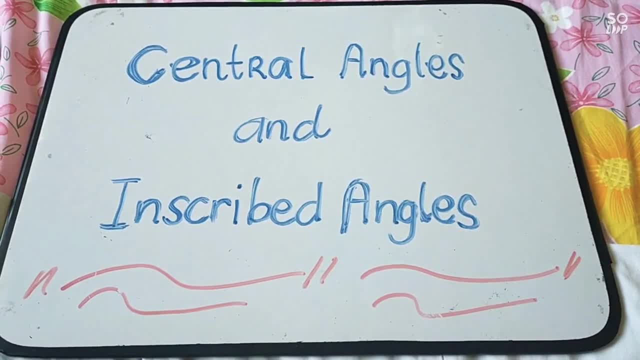 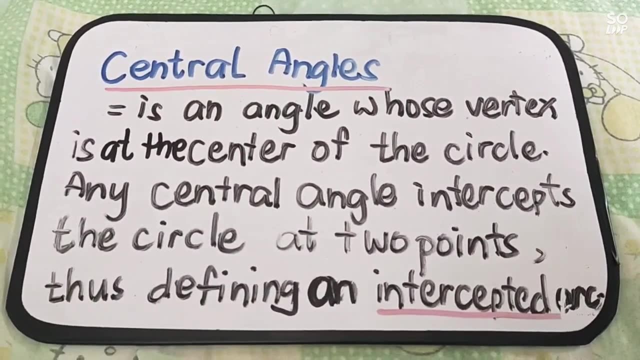 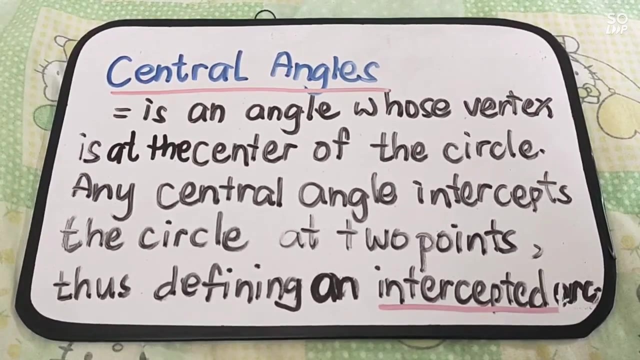 Hi guys, our topic for today is about central angles and inscribed angles. Let us define central angles. Central angles is an angle whose vertex is at the center of the circle and its central angle intercept the circle at two points, thus defining an intercepted arc. 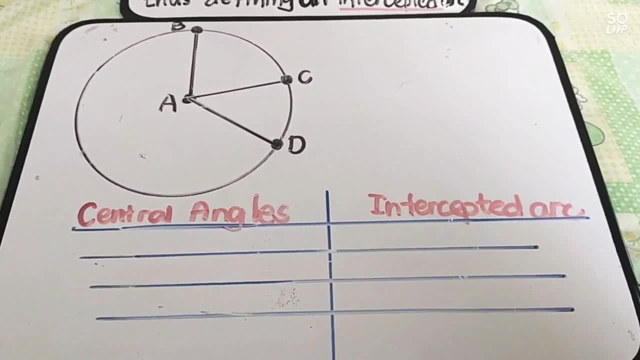 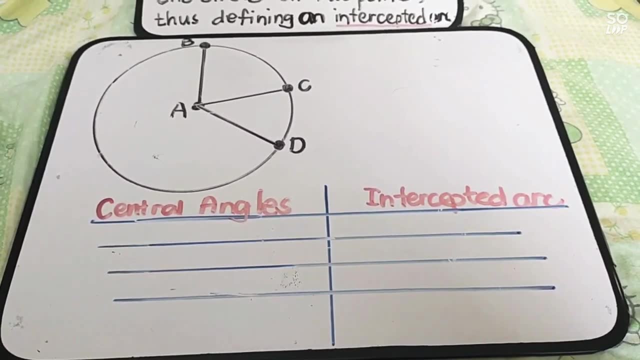 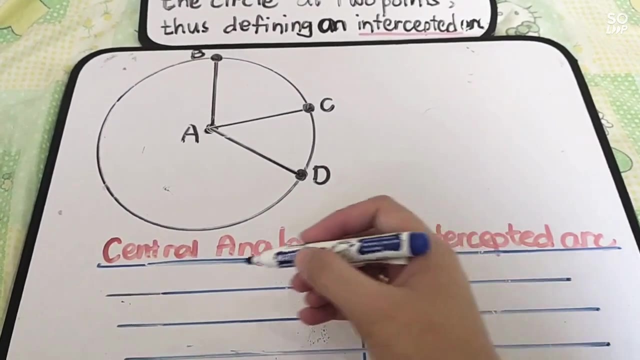 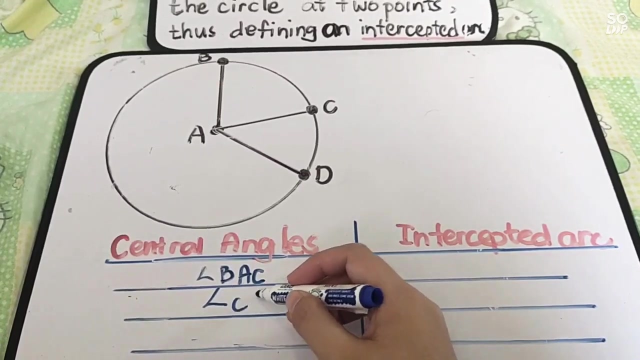 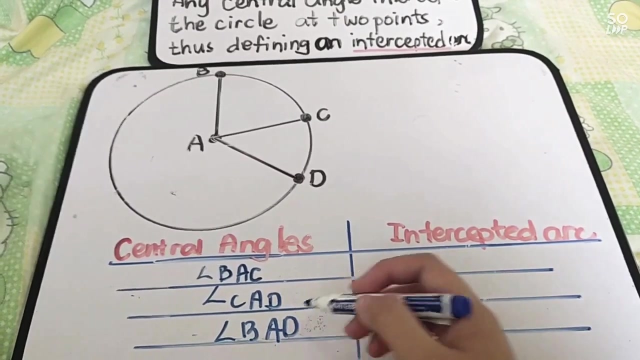 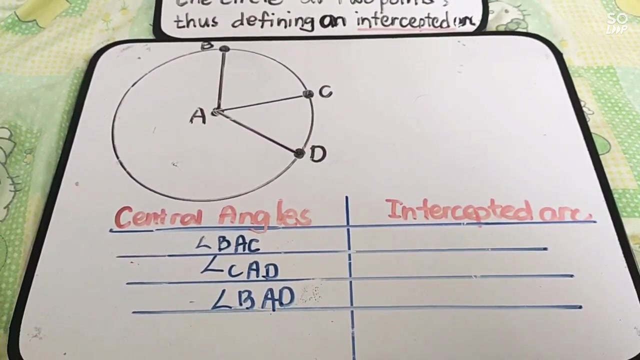 Let's have an example. Consider circle A. Let us determine in the circle A what are the central angles and its intercepted arc. Let us name all the central angles. We have angle BAC, angle CAD and angle BAD. Those are the central angles that you can see in the given figure. Now let's name the intercepted. 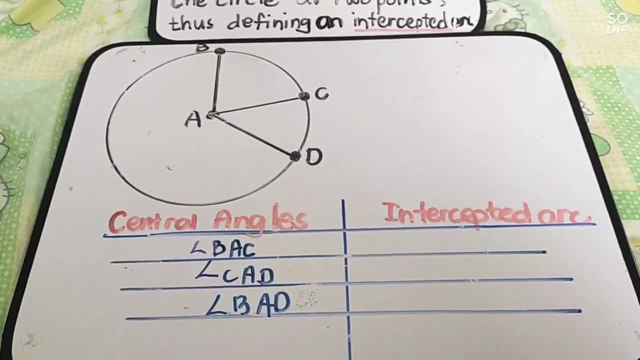 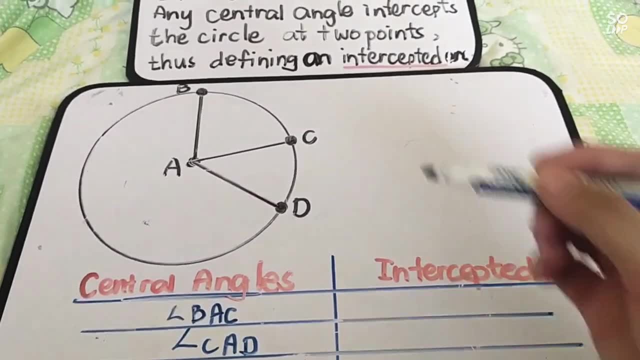 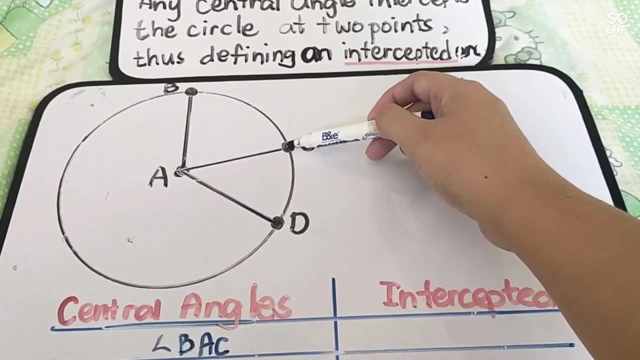 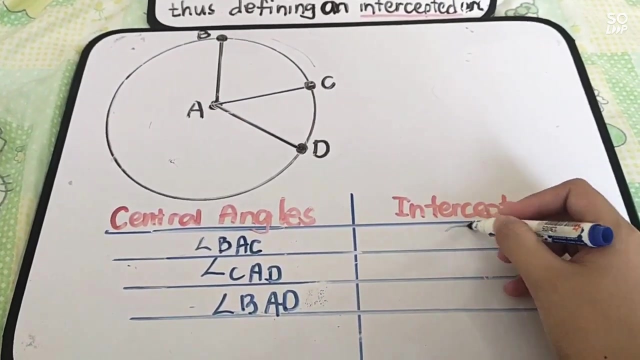 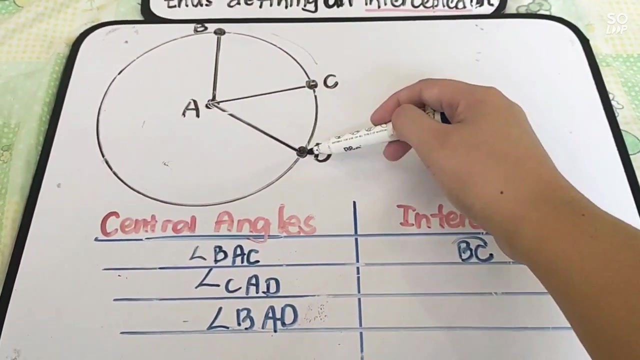 arc, The intercepted arc. this is the arc that formed by the angles, by the central angles. Okay, if this is an angle BAC, then this is the arc that formed by angle BAC. So what arc is it? So we have arc BC, Arc BC. Next, we have angle CAD. So the arc formed by CAD is this arc. 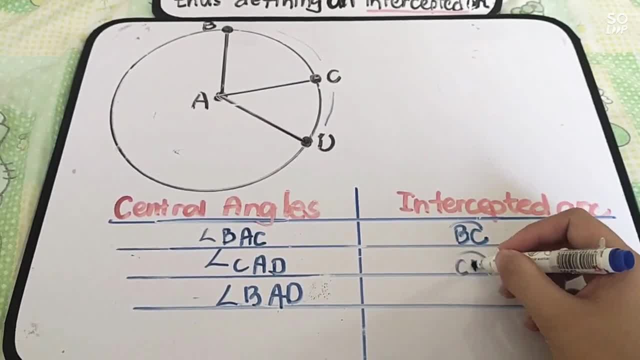 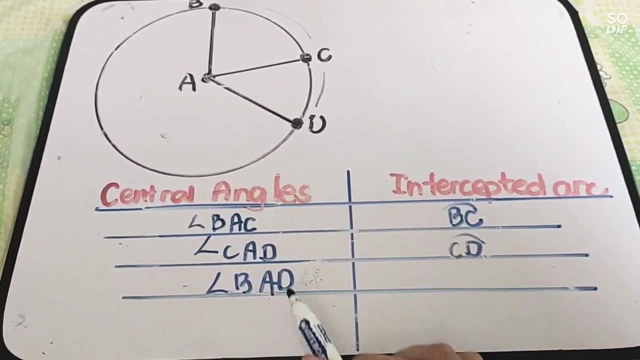 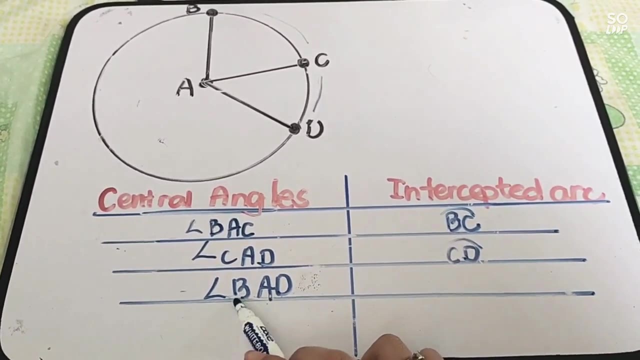 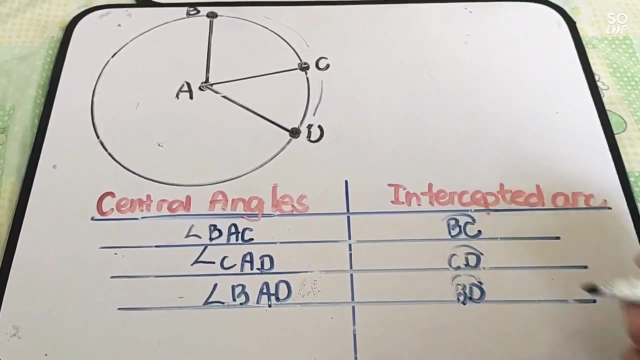 So we have arc CD. As you observe, when you are going to find the intercepted arc of the central angles, the vertex will disappear. So therefore, if we have angle BAD, therefore its intercepted arc is arc BD. Okay, next we have 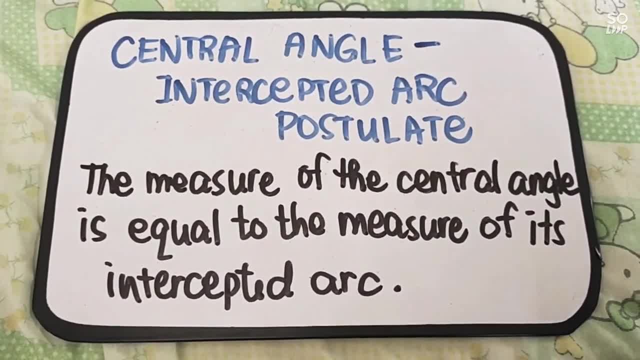 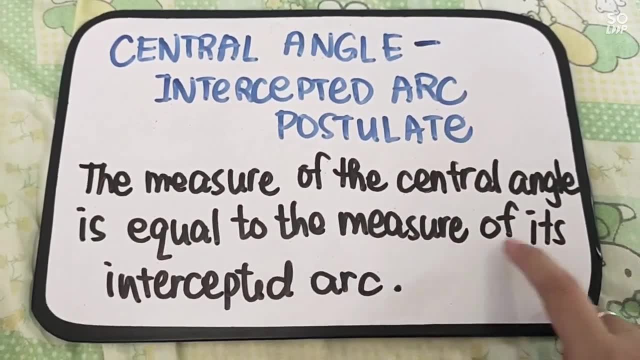 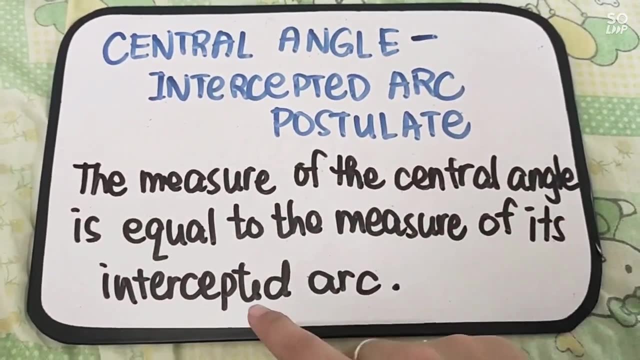 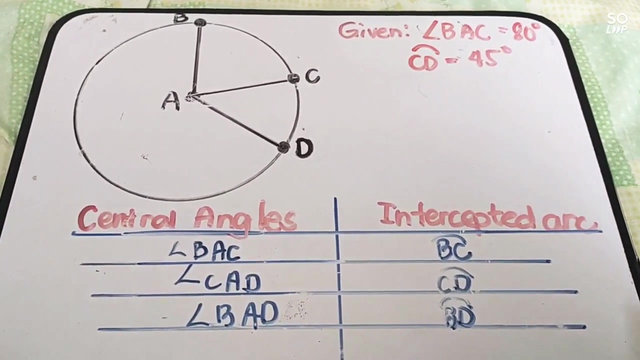 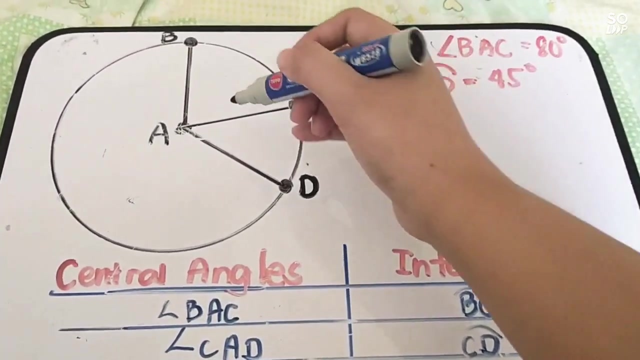 what you called central angle intercepted arc postulate. It says that the measure of the central angle is equal to the measure of its intercepted arc. Take note: central angle is equal to its intercepted arc. consider again this figure, circle a, we have a given of angle. bac is equals to 80, 80 degree. so this one is 80 degree. the angle then arc, cd is: 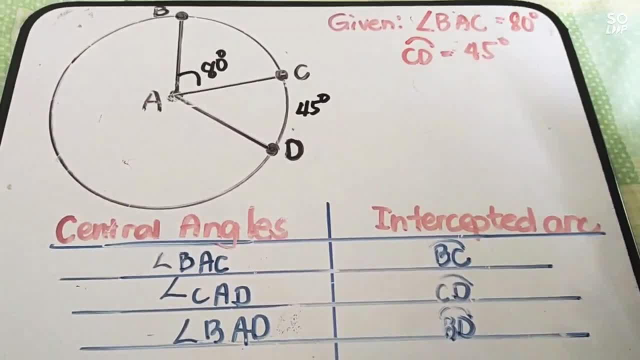 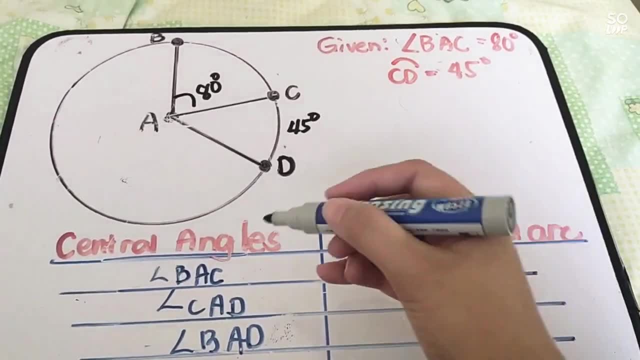 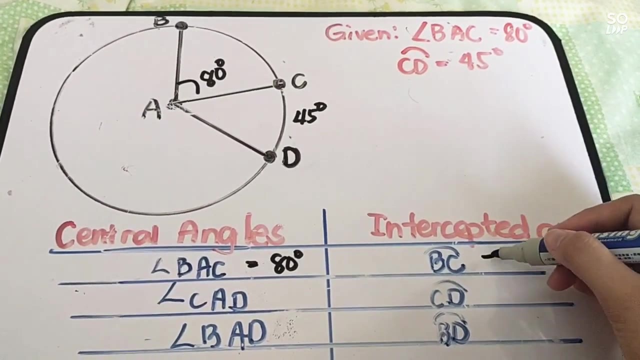 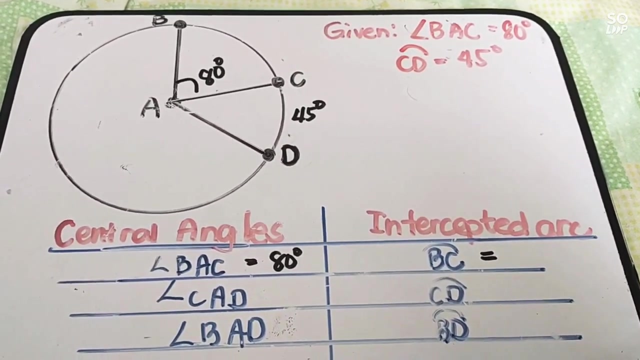 equals to 45 degree. let us find the other measurement of the following angles and intercepted arc. so it says that bac is equals to 80 degrees. then how about the its intercepted arc? again in central angle. intercepted arc postulates central angle is equal to the measure of its. 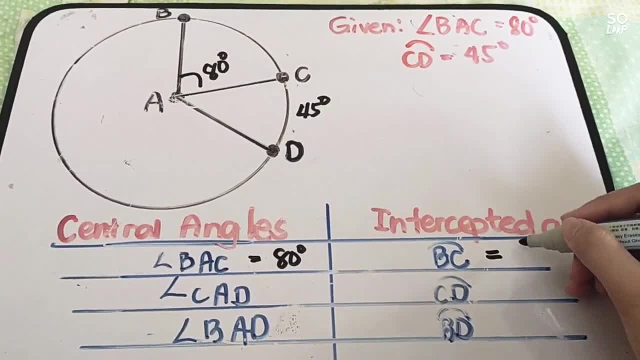 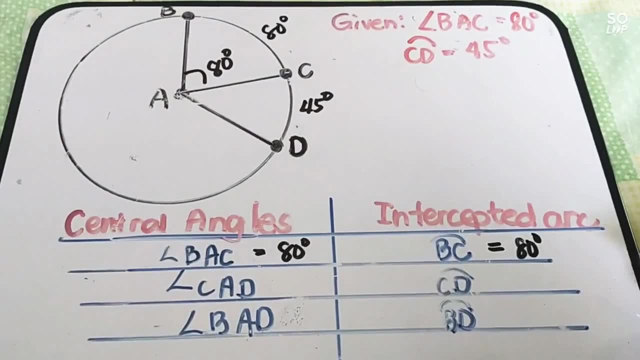 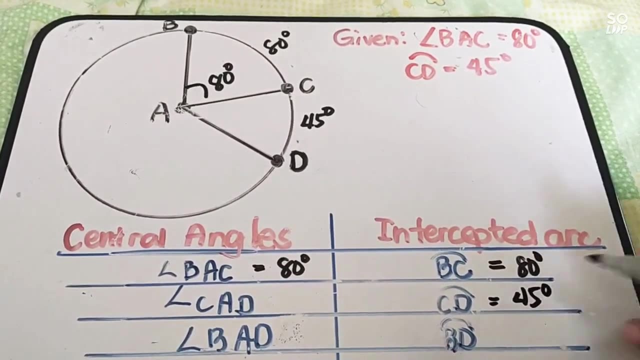 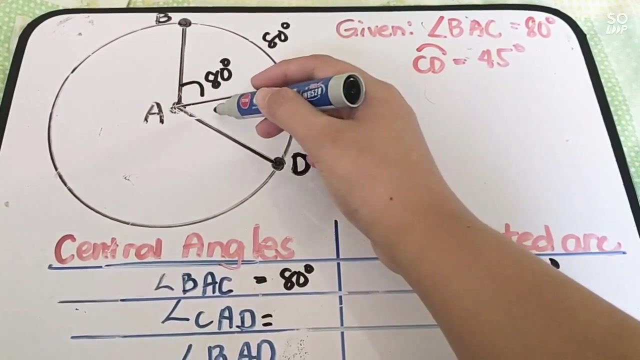 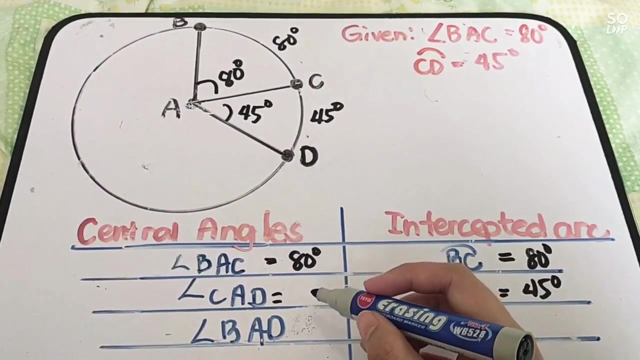 intercepted arc. therefore, arc bc is also 80 degrees. so therefore this one is 80 degrees. next we have arc cd. arc cd is 45 degrees. therefore, what's the measurement of angle cad? all right, it is also 45 degrees by using, again, central angle intercepted arc. 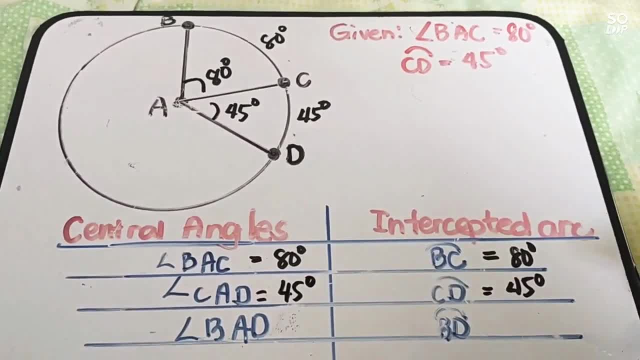 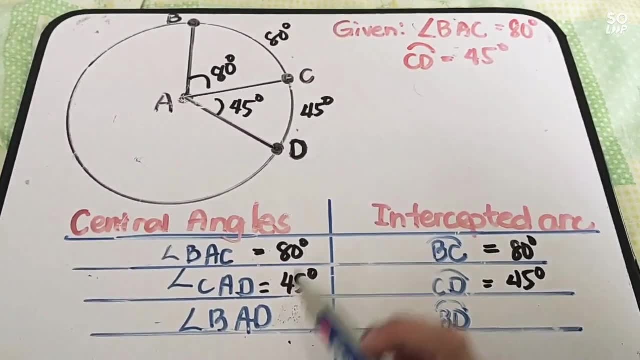 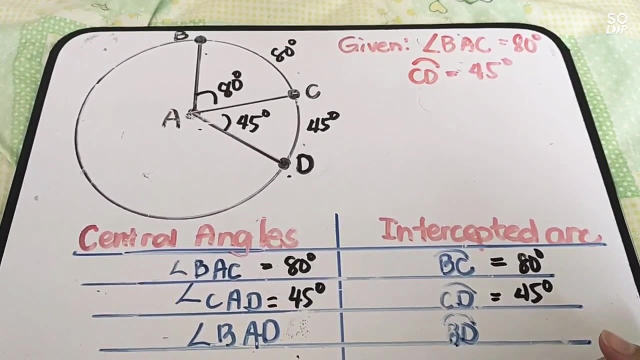 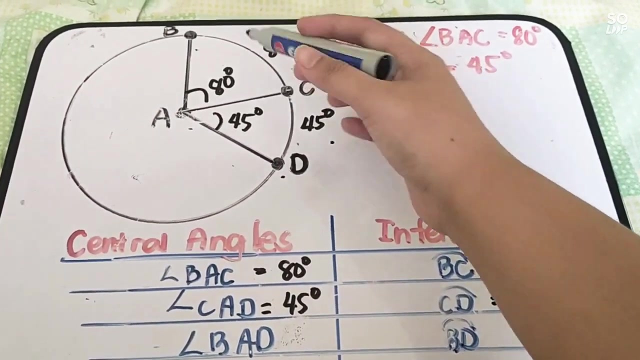 so this is exactly what we are going to postulate. this is 45 degrees. okay, next, what is the measurement of angle bad, b a d? how would you find bad? so this time you are going to add 80 plus 45 for us to find the angle b a d. 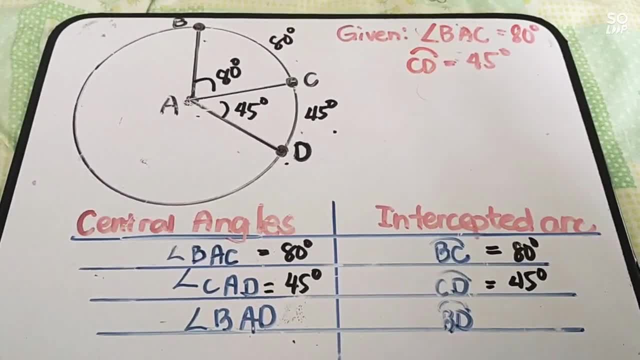 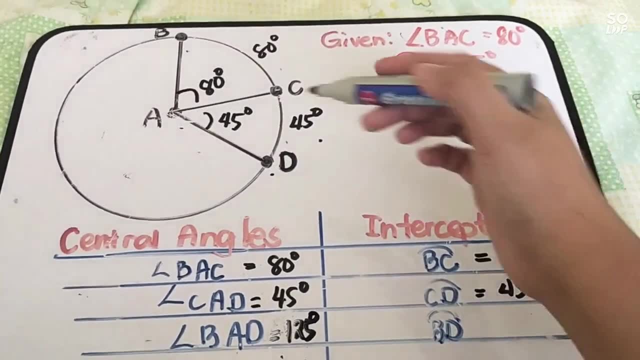 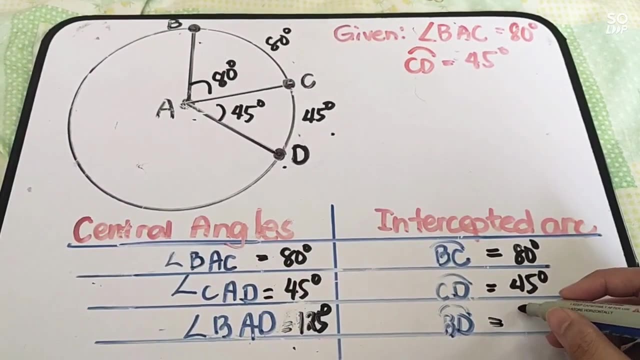 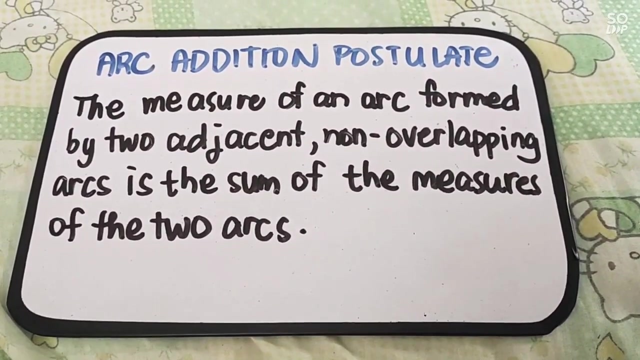 now, what is 80 plus 45? 45 degrees. So the answer is 125 degrees. If BAD is 125 degrees, therefore arc BD is also 125 degrees. Let's move with arc addition postulate. It says that the measure of an 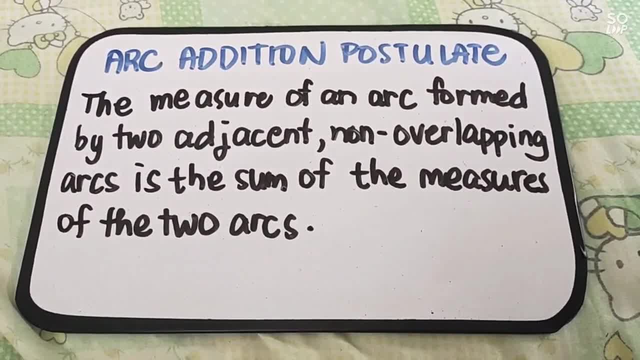 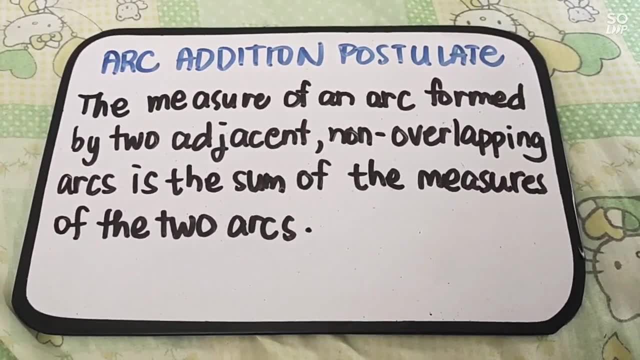 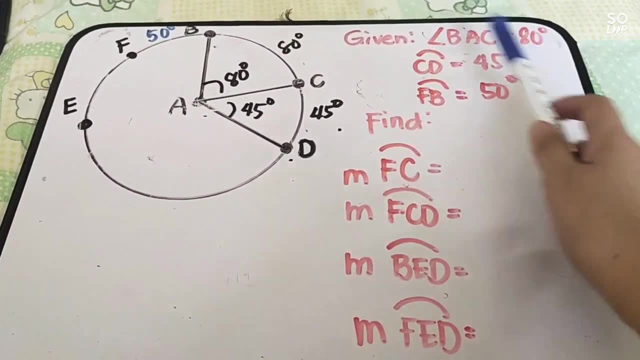 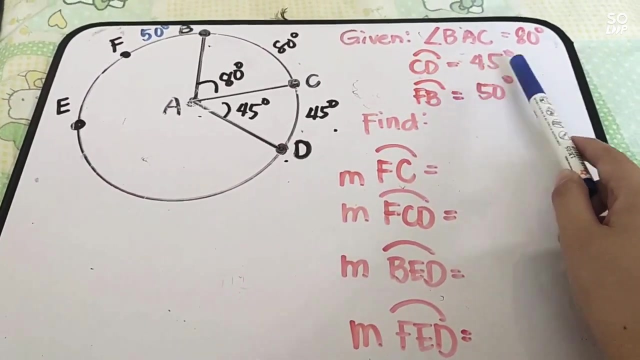 arc formed by two adjacent, non-overlapping arcs is the sum of the measures of the two arcs. Let's have an example. Consider the circle A. We have a given of arc. BAC is equal to 80 degrees. therefore the intercepted arc is also 80 degrees. We have arc CD, which is: 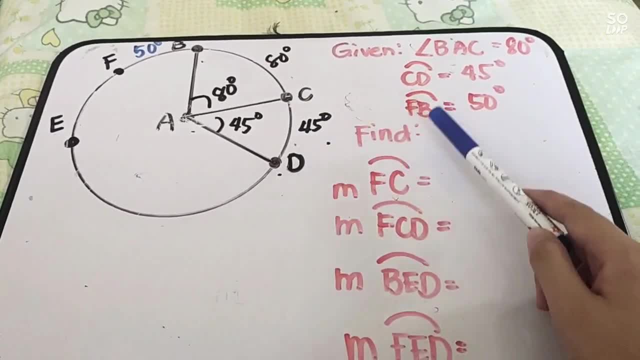 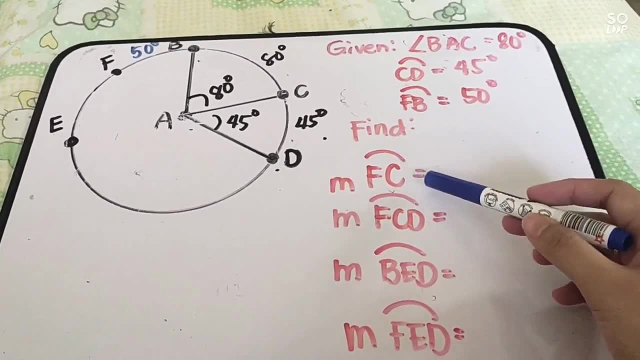 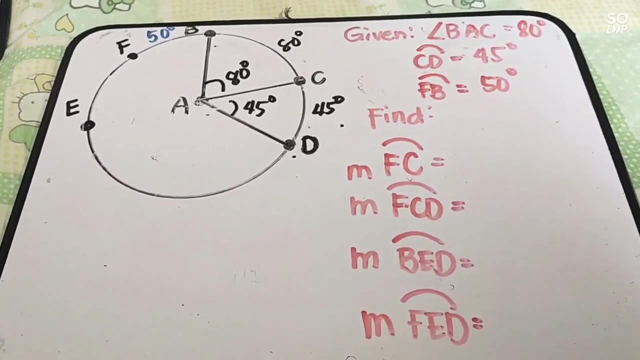 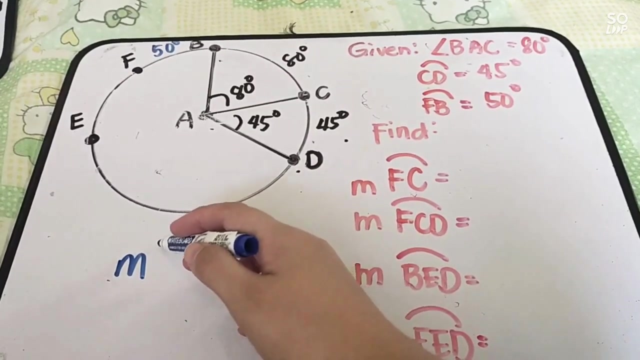 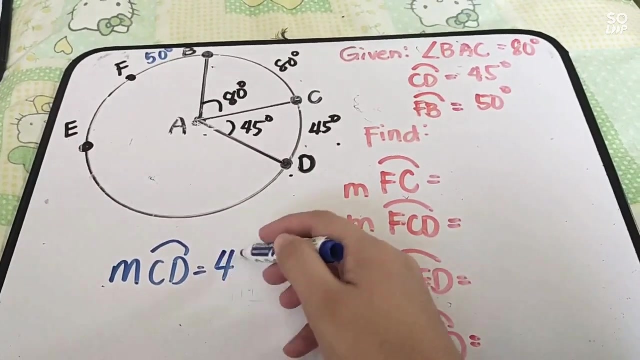 45 degrees here and then arc FB. We are going to find for the measure of FB, FCD, BED and FED. Take note class. if the given has letter M on the side, or measure arc CD, your answer should have no degree. 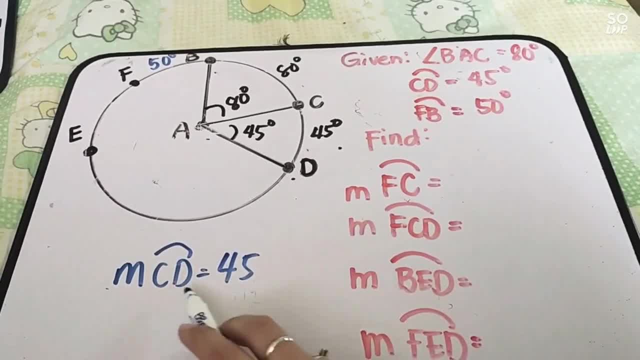 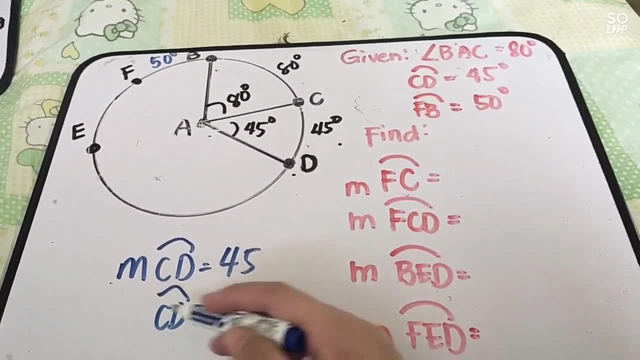 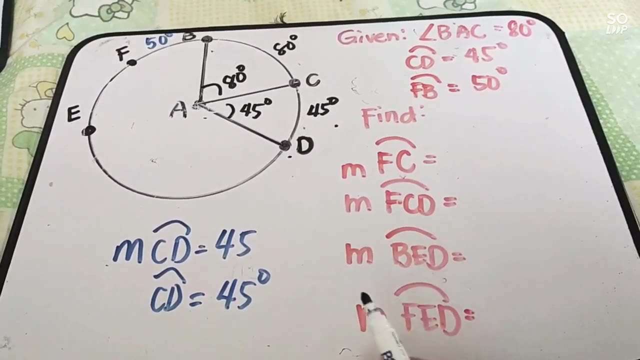 sign We have measure of arc CD is equal to 45. If we are only looking for arc CD and there is no measurement, we have 45 degrees. Is it clear? So, since we are looking for a measure or letter M on the 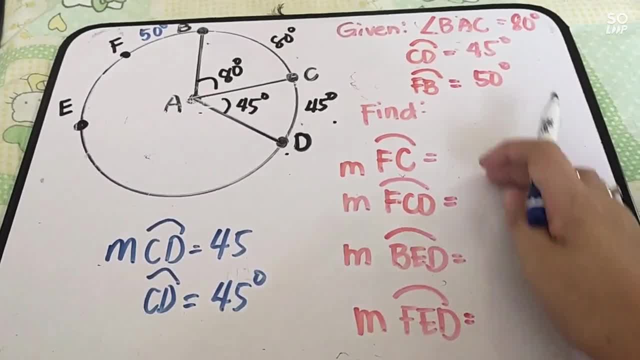 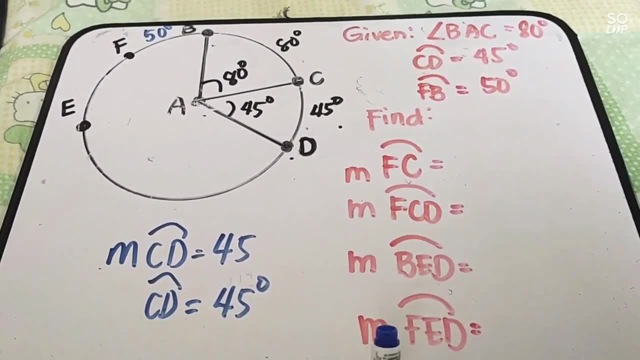 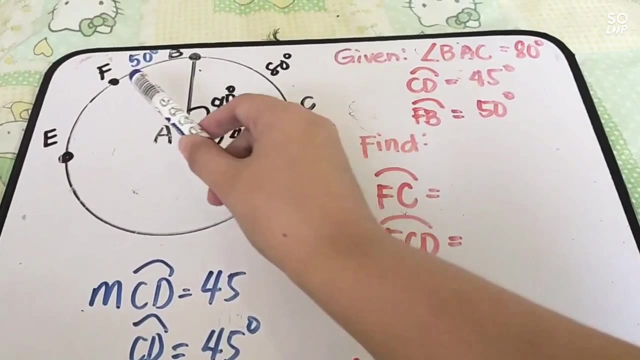 side. therefore, your answer here is: there is no degree sign. Is it clear? Okay, now let us answer arc FC- Measure of arc FC. If we need to find for the measure of arc FC, this one, So we need to add the measurement. of FB and BC. So we have 50 plus, or equal to 3,. therefore C circle H is equal or congruent to circle I. So that is what you call congruent circle. The radii to both circles are just the same. Okay, let's have example of congruent arcs. We have a given here of circle H and circle I. Let us have for a circle H. It says that we have here a given of SHI, which are 60 degrees, and then an arc here which is arc LR, which is also 60 degrees. According to congruent arcs, arcs would have the same measurement. So, since this one is a central angle, therefore this arc is also 60 degrees. Okay then, since this one is an arc of 60 degrees, therefore this central angle is also 60 degrees. And take note class. kapag siya po ay nagkaroon ng vertical angles like this one. this one is what you call a vertical angles. They are always equal or the same. Okay, then this one is a straight line. Kung ito ay straight line, para makuha mo yung kabilang side niya. a straight line is always 180 degrees. So meron ka ng 60, para makuha mo yung kabilang side, subrak mo lang siya sa 180, that is 120 degrees, And this one vertical ulit. ito therefore 120 degrees. Okay, then this one. vertical ulit ito, therefore 120 degrees. Okay, then this one vertical ulit ito, therefore 120 degrees din ito. So, since ito ay central angle, this arc is also 120 and this one is also 120 degrees. Ganun lang kumuha ng mga arcs and angles. Kapag yung given mo is a central angles or we have a vertical angles, Is it clear? Next tayo, We have this one, This one, wala ka ditong vertical angles, Kung makikita mo. Nakia ko dal 65 toes, but yung nakaka-cook na makinig Ito, kung makikita mo, hindi naman syo is nagkaroon na create ng cross talaga sa line or a straight line, Kasi dito sa kabilang side dumaan sya sa diameter eh. bento yung vertigo retreat magiging lang. This one wala wala kang diameter dito, Puro radius lang. So since this one is 70 degrees, therefore ar is also 70 degrees, And then and RQP is 70, therefore angle QIP. this one is also 70 degrees. So since this one is 70 degrees, therefore RQP is 70 degrees, And then angle: RQP is 70, therefore angle, QIP, this one is also 70 degrees, also 70 degrees. So ang tinatawag natin congruent arcs here is the OR, at saka CQP. okay, That is. congruent arcs. Let's move with theorems on arcs, chords and central angles. It says that if two central angles are congruent, then the corresponding minor arc are also congruent, And if two central angles are congruent, then the corresponding chords are also congruent. Let us have an example. Let us consider again circle H and circle I here. So nagdagdag lang ako ng chord: Okay, sabi doon sa kanina sabi niya, if two central angles are congruent, then the corresponding minor arc are also congruent. So therefore, if we have a central angle here, and then this is the corresponding minor arc, then the corresponding minor arc is also congruent. So therefore, if we have a central angle here and then this is the corresponding minor arc, then the corresponding arc, they are also congruent. So meaning: si angle, SHI is congruent to angle. we have RHL Ayan. Then ang corresponding arc ni SHI ay si arc. SI this one is congruent to arc LR or RL Ayan, So yun yung ibig sabihin nung unang teorem. Yun sa pangalawang teorem naman sabi niya: if two central angles are: 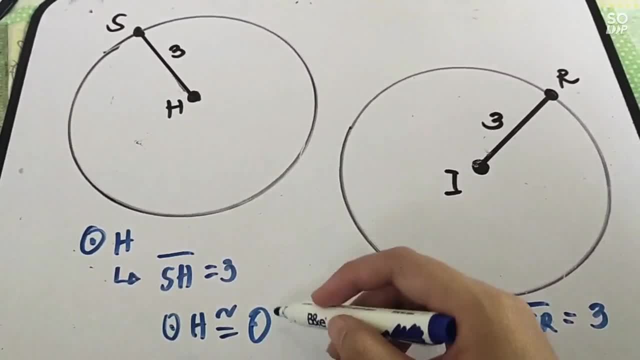 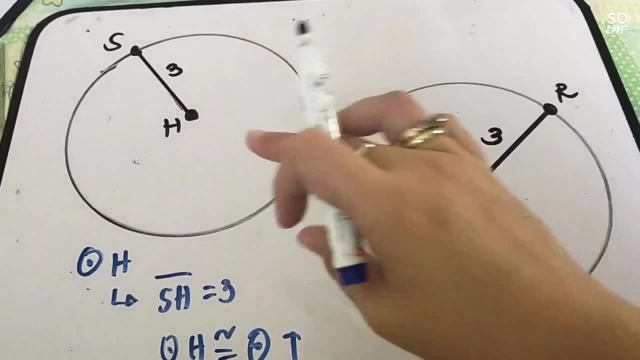 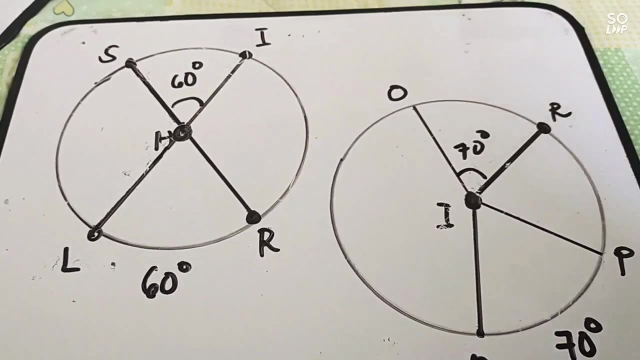 congruent, then the corresponding chords are also congruent. So naglagay ako dito ng chord, dun sa same central angles here. So dito we have a chord here. ang measurement niya ay 3.. So since nasa central 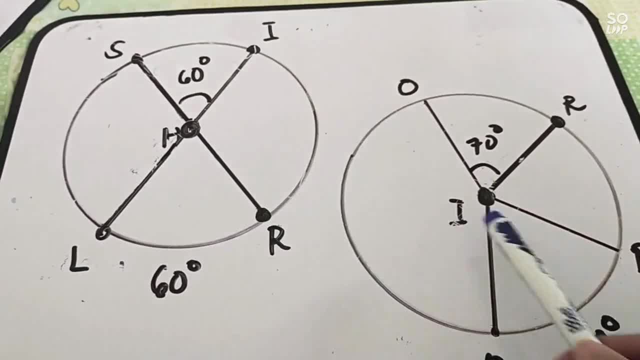 angles, siya at parehas, siya yung kanyang sukat, therefore yung measurement niya ay 3.. So, since nasa central angles, siya at parehas, siya yung kanyang sukat, therefore yung measurement niya ay 3.. 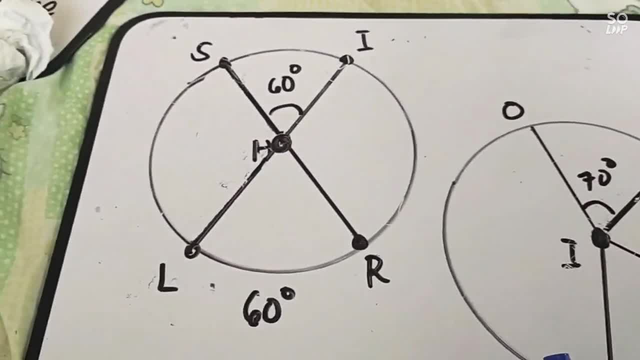 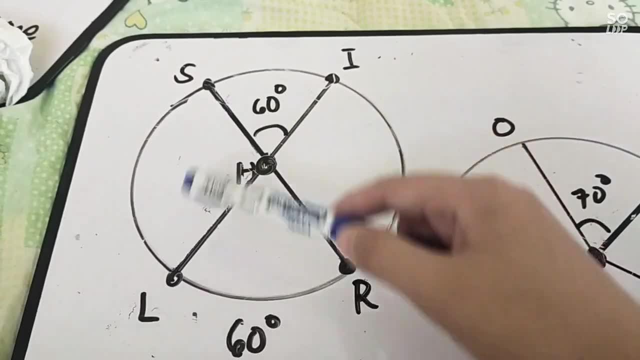 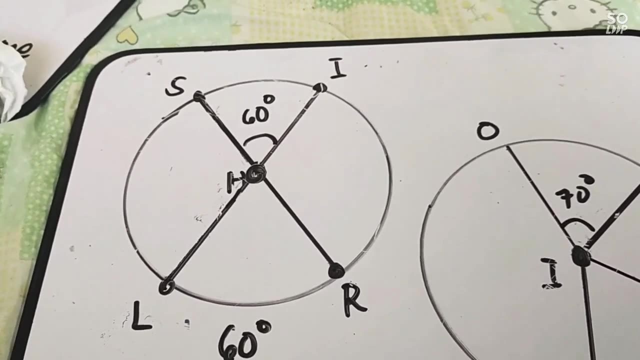 measurement here of this cord SI is also 3.. Meaning the line segment SI is congruent to line segment LR. That's it, Okay. So this one. Let's go next. We have here circle I. It says here: this measurement is 4.. 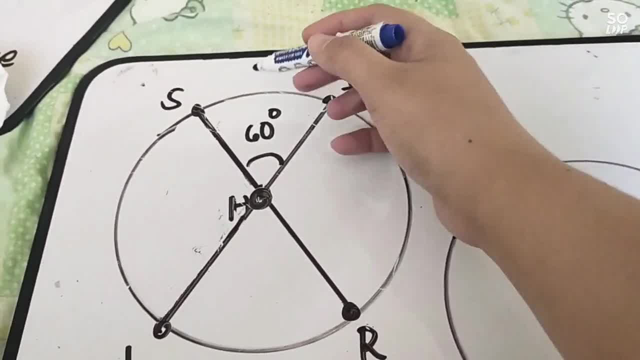 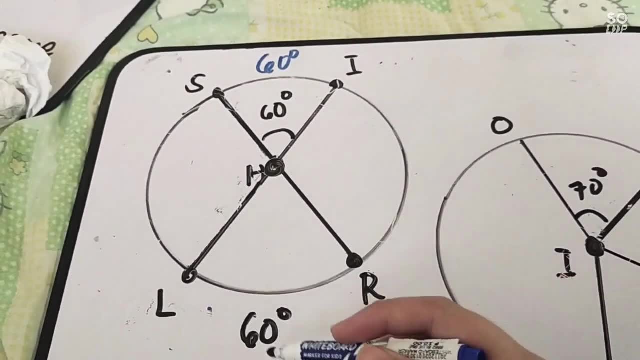 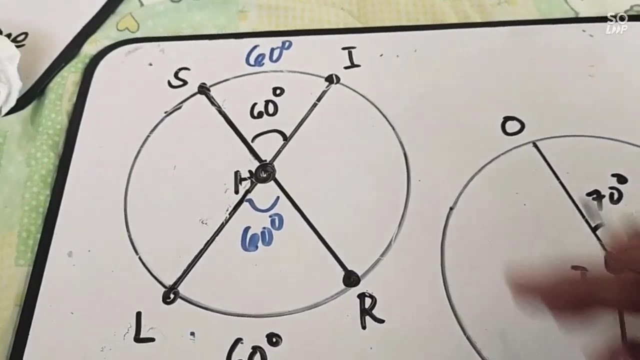 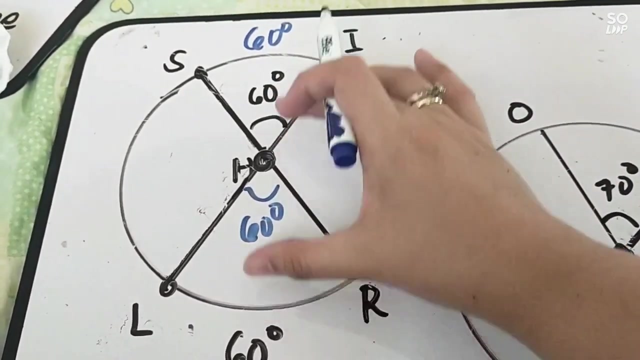 And the central angles are congruent. Therefore, the missing cord here is also 4.. Okay, So COR is congruent to line segment QP. They have the same measurement. Is it clear? Let's have this figure. We have a given of PQ or arc. PQ is 2x minus 10 and arc QR is equal to x plus 40.. 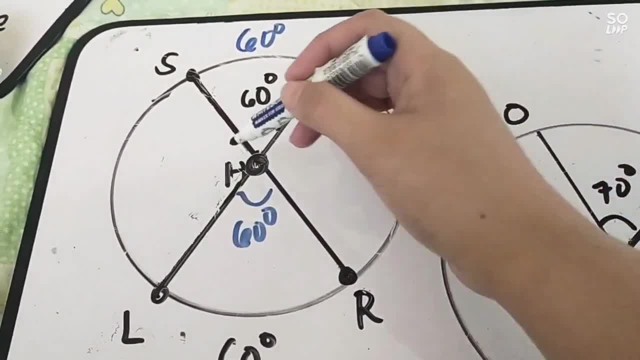 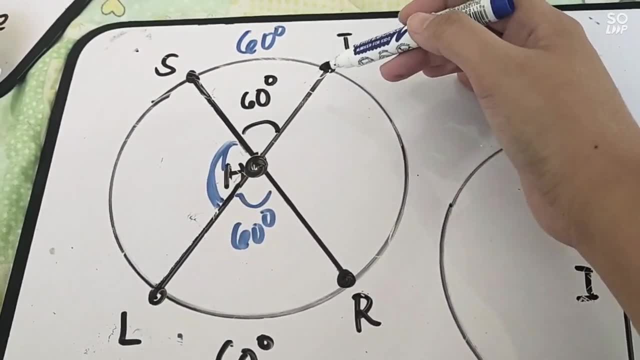 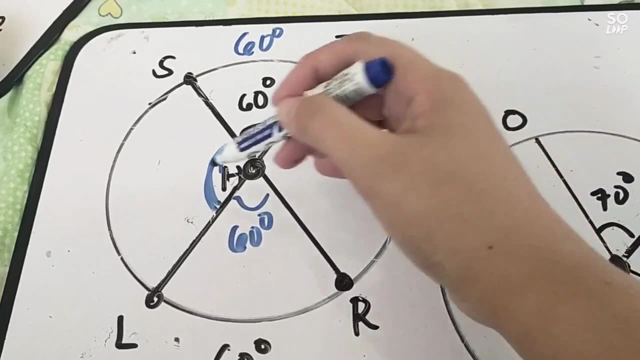 Let us find x arc PQ and arc QR. It says that it said earlier. we have the. if we have congruent central angles, therefore its arc is also congruent. So since this one is 90, and this is a semicircle, therefore this is also 90.. 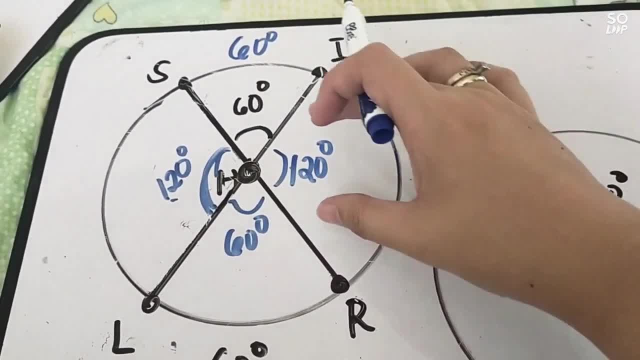 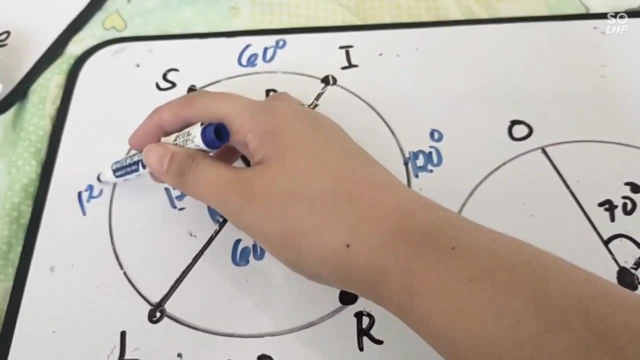 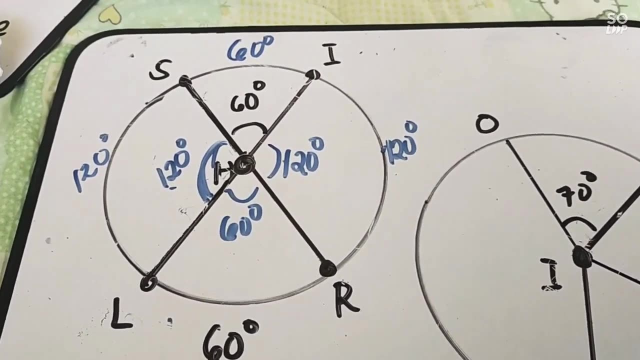 This is also 90 degrees. This is also 90 degrees There. So for us to see, To solve for x, they are equal. So therefore 2x minus 10 is equal to x plus 40. Then transposition lang to solve for x, So you have 2x lipat mo. yung x to the other side becomes minus x. 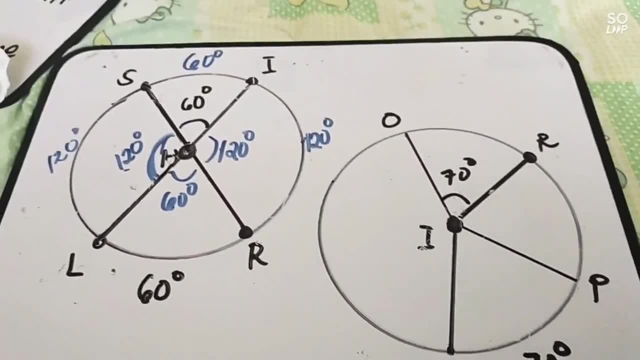 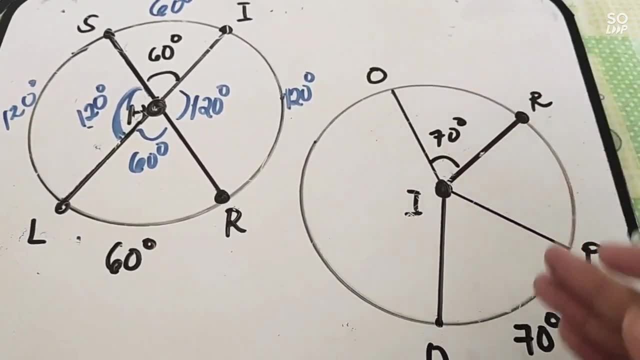 Just change the sign, Then copy 40 here, Then si 10 naman, lipat mo sa kabilang side, it becomes plus 10.. So 2x minus x, we have here x is equal to 50.. 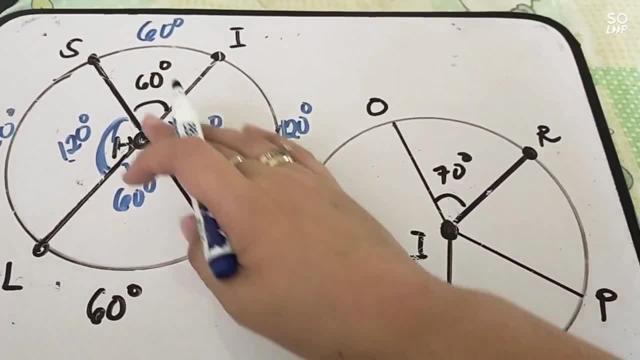 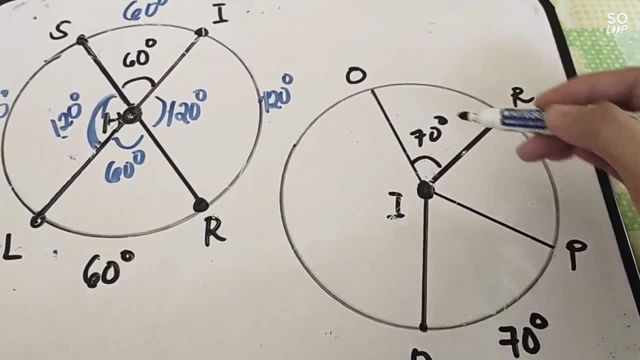 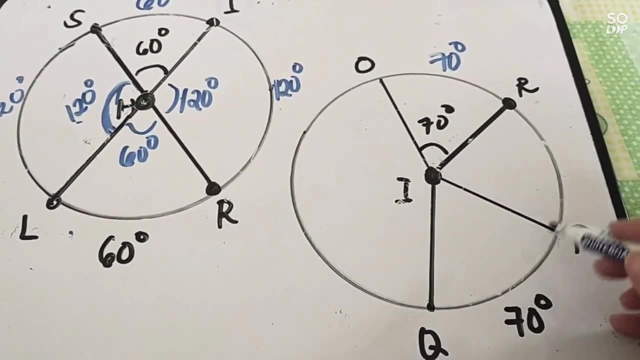 So this is your x. Now we are going to substitute that Kailangan. ang maging sagot nya is 90.. We have arc. PQ is equal to 2x minus 10.. So we have 2 times 50 minus 10.. 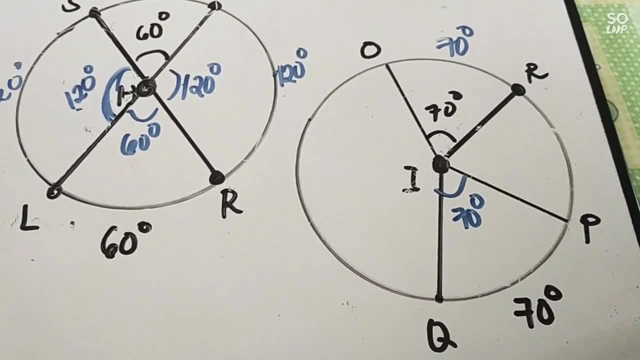 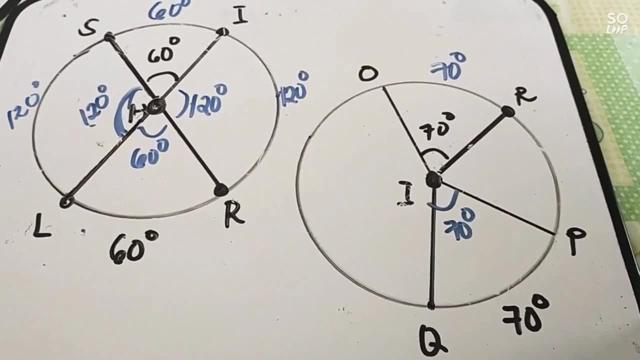 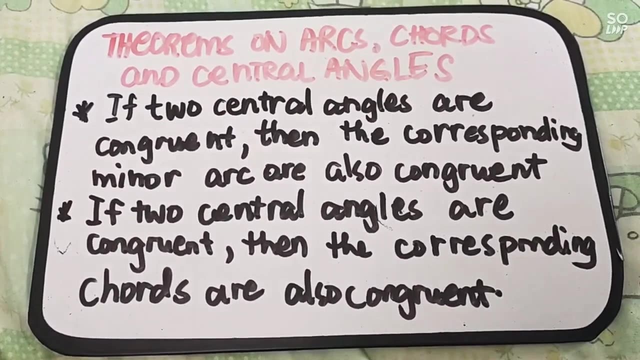 So 2 times 50, we have here 100 minus 10.. The answer is 90.. Okay, 90 degrees, Is it clear? Next, yung isa din. we have arc QR. Si arc QR ay equal sya kay x plus 40.. 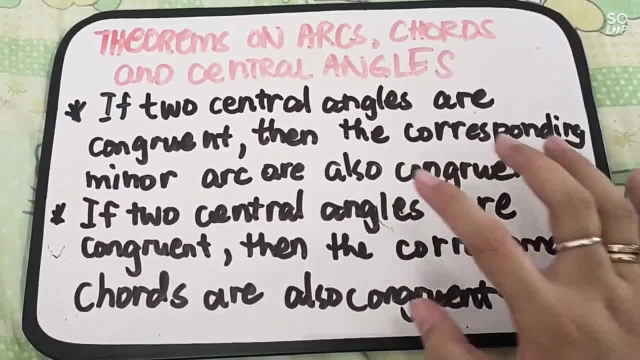 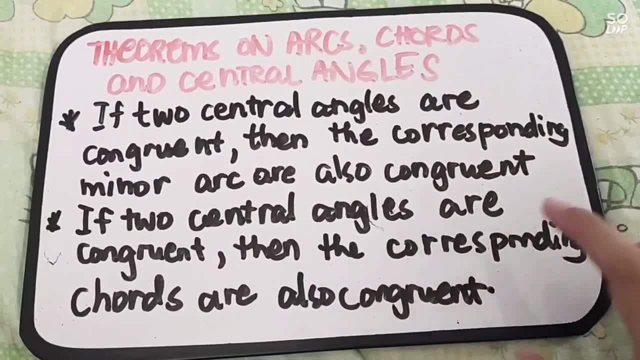 So we have here 50 plus 40. The answer here is 90 degrees. Is it clear? Gumamit ako ng degree sign, kasi wala naman akong letter M. Pero kung may letter M ako dyan, pwede na akong hindi gumamit ng degree sign. 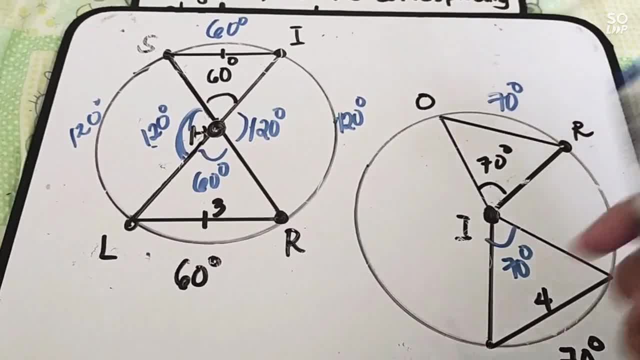 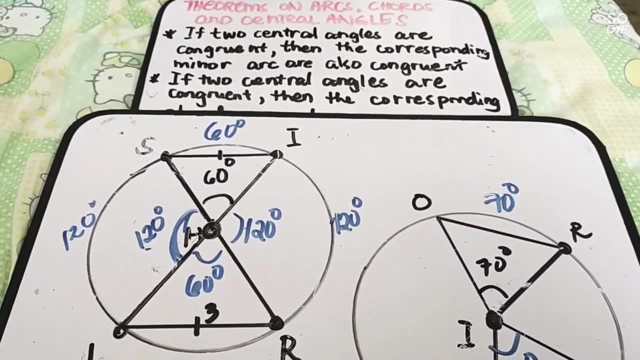 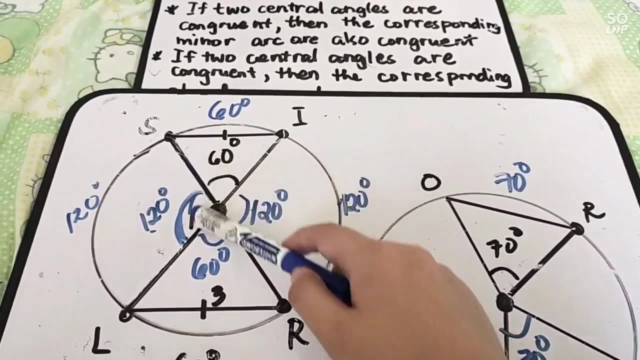 Okay, Let's move with inscribed angles. So inscribed angle is an angle whose vertex lies on the circle and whose sides contain chords of the circle. So meron tayong tatlong case naman ni 100.. The answer now is 50 degrees. 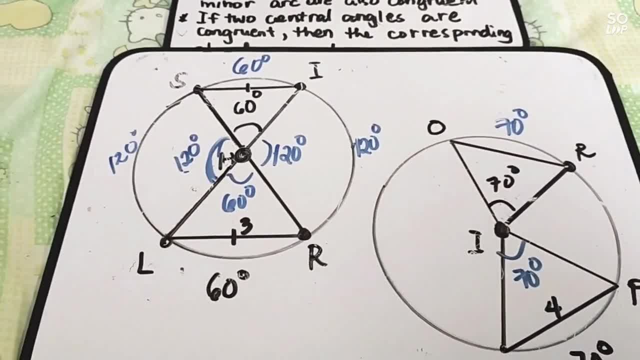 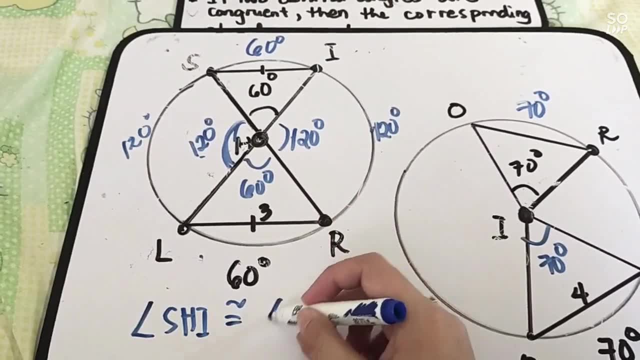 Ganun lang po kasimple si inscribed at saka si intercepted arc. Next this one: Si angle HGI daw po, Si angle PQT daw po is 30 degrees. Okay, now what's the measurement of HI? 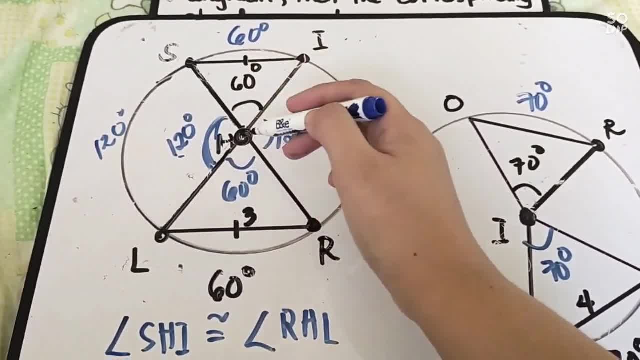 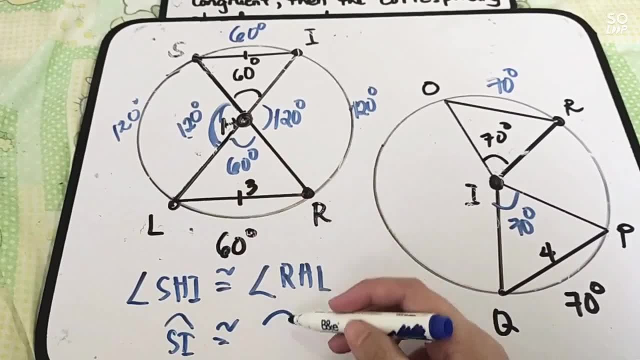 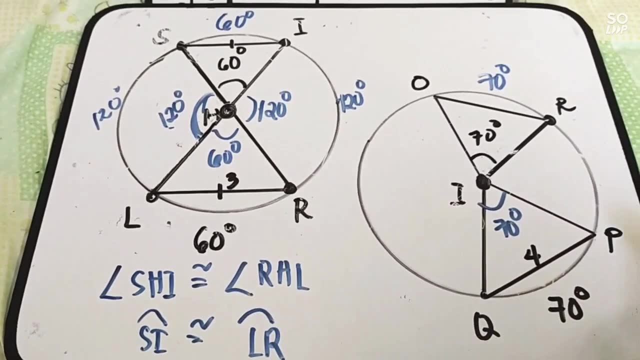 So, multiplied by 2, the answer is 60 degrees. So HI is equal to 60 degrees. Is it clear? Let's have another example. Consider circle O here. Okay, we have a given of measure of angle. PQT is 80.. 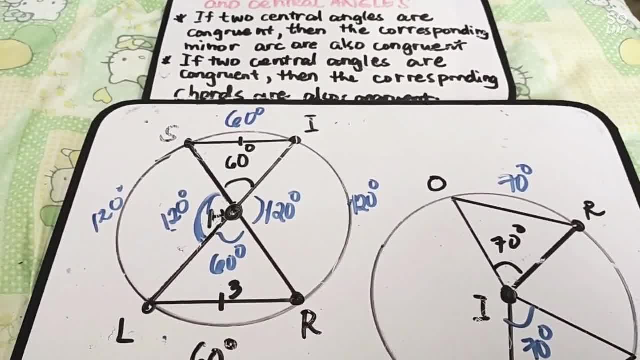 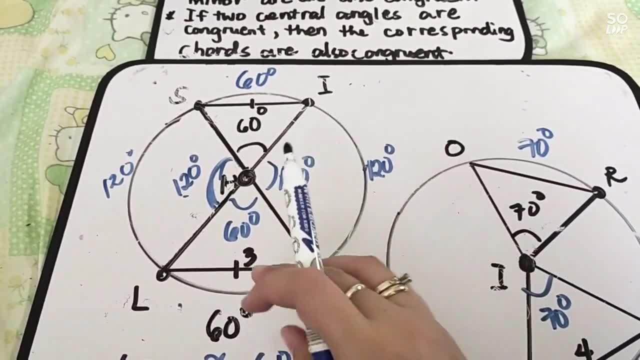 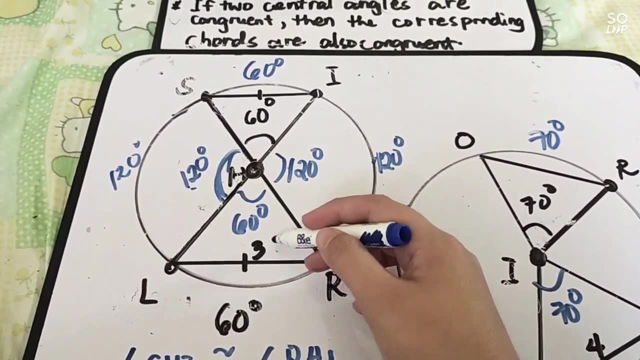 Si PQT daw po is 80 degrees. Okay, so dito hindi lang ng degree kasi may measurement naman Then, measure of angle ST. arc ST is equal to 30 degrees. We are going to find for the arc PT and measure of angle of PRS. 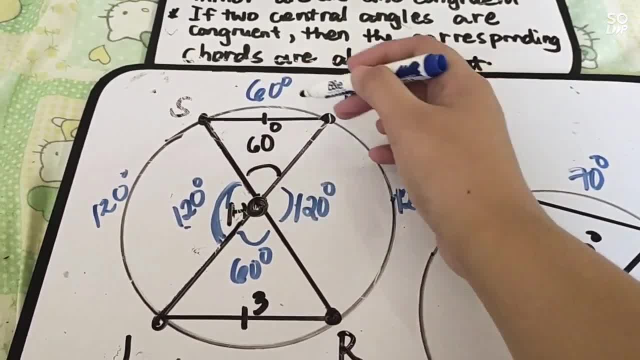 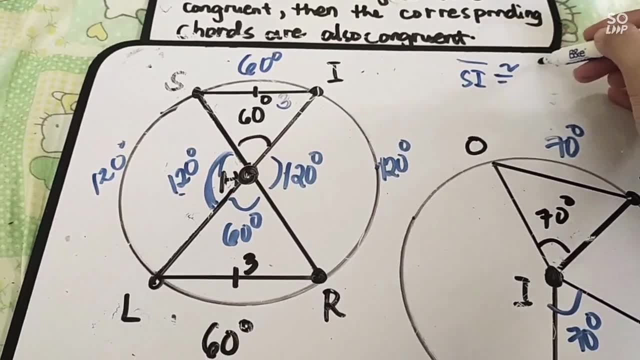 Tingnan nyo po, ah. So, since this one is an inscribed angle, PQT is an inscribed etong nabuo niyang arc. ang kanyang intercepted arc, therefore, is twice ng kanyang inscribed angle. 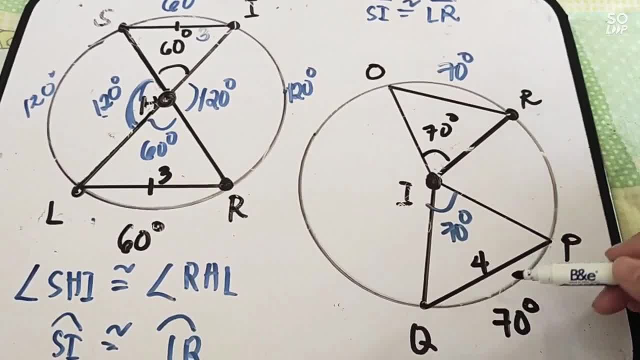 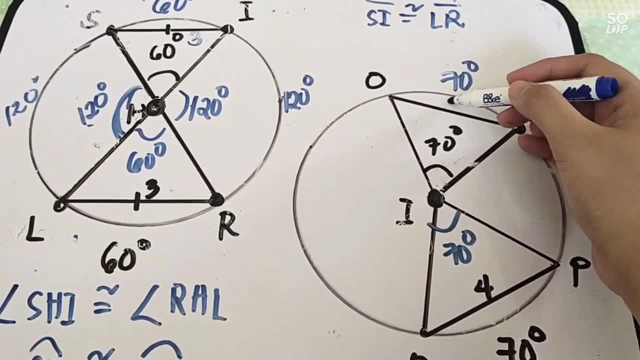 So 80 times 2, this is 160 degrees. Okay, so, bago kayo magsagot, dito dito muna kayo, I-analyze nyo muna yung circle. Next tayo Dito tayo: 30 degrees. 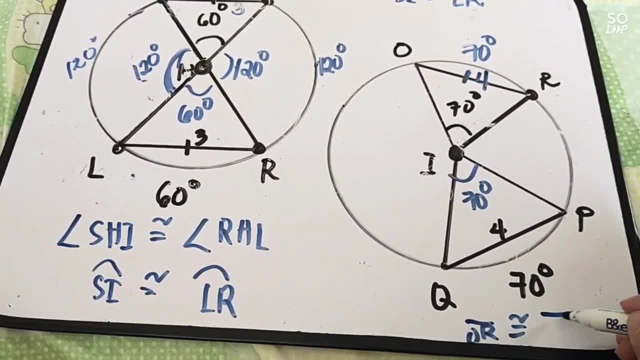 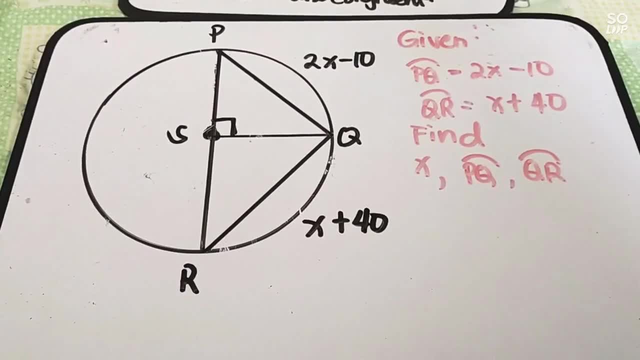 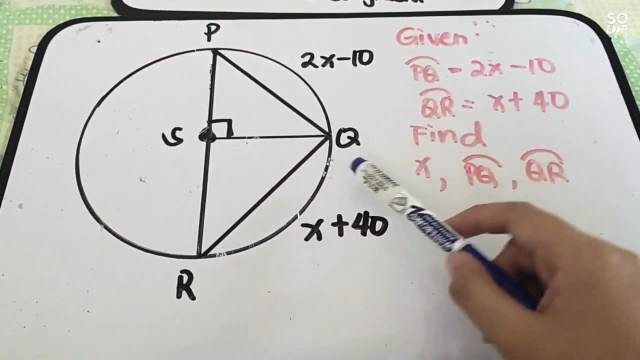 Eto CST daw, Eto daw pong CST. So let us analyze Kung paano natin makukuha si PRS. As you can see, guys, si PRS ay inscribed angle, Then ang kanyang intercepted arc etong buo na to na si PS. 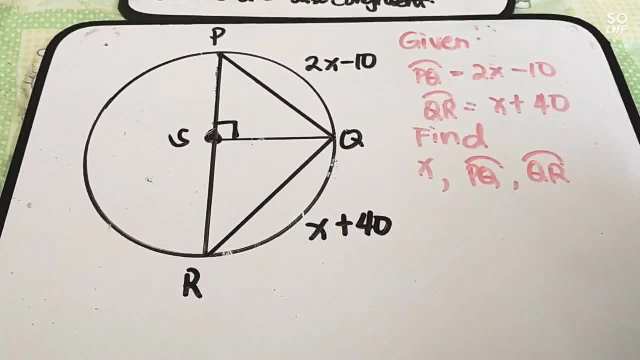 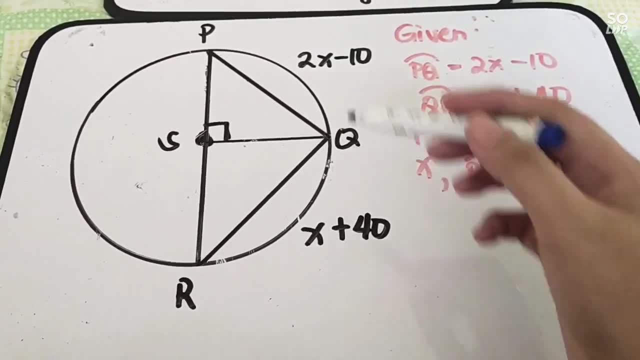 Okay, So si PT raw ay 160, then si TS ay 30.. Therefore, ilan ngayon si PS. So, kung mapapansin mo, si PS ay magiging na siyang 160 plus. 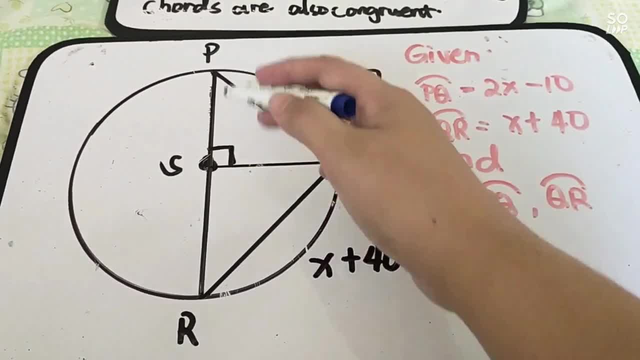 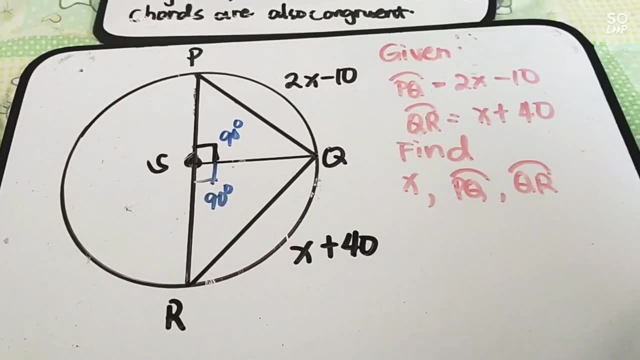 30,. the answer is 190 degrees. Did you get it? So gumamit naman tayo ng arc addition postulate dyan. Okay, So nakukuha na natin yung kanyang intercepted arc. therefore. 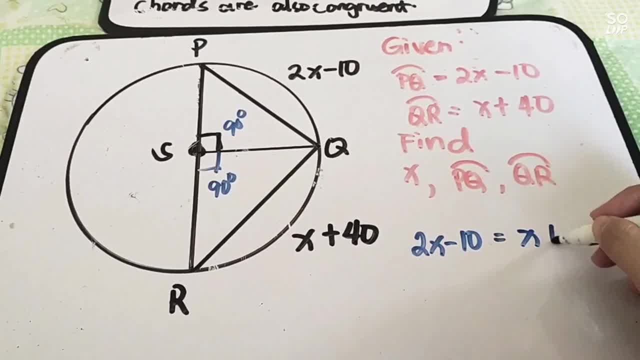 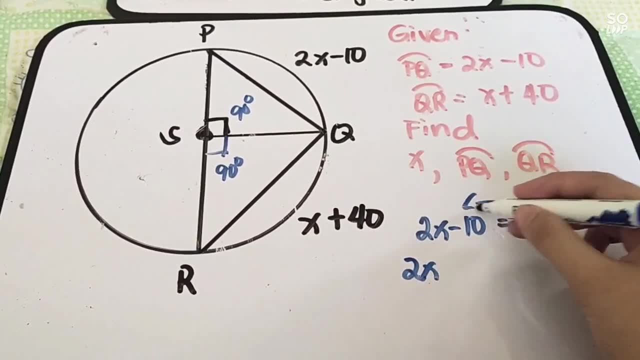 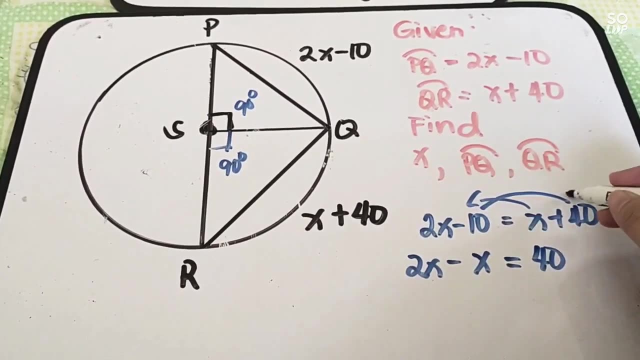 let us find the inscribed angle by divide 190 into 2.. So the answer is 95 degrees: 95 degrees. So arc PS is 190.. When you divide it into 2, the answer is 95 degrees. 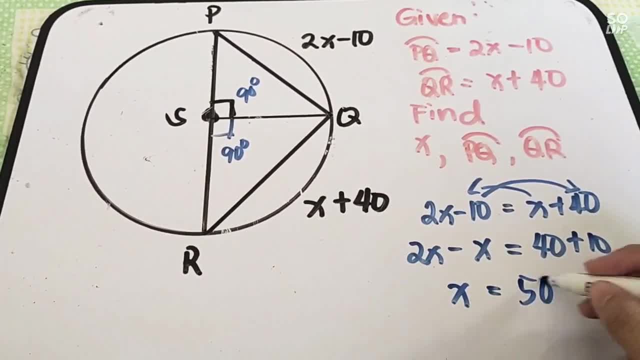 This is now your angle. PRS. Is it clear? So 95 degrees.